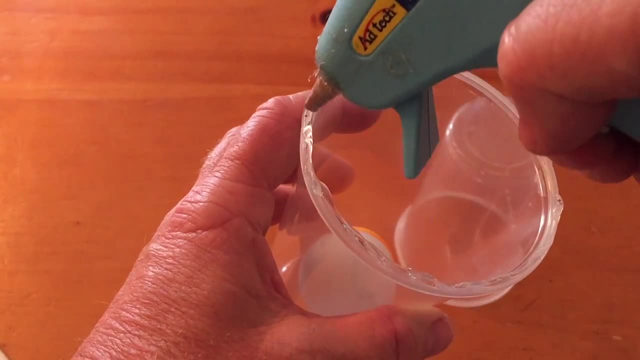 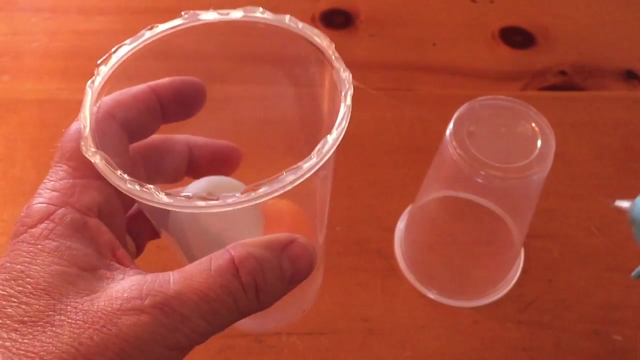 Go all the way around on the outside top of the cup rim right here. When you get completely all the way down with the glue, then you're going to take the other cup and you're going to seal it off by just putting it on top. 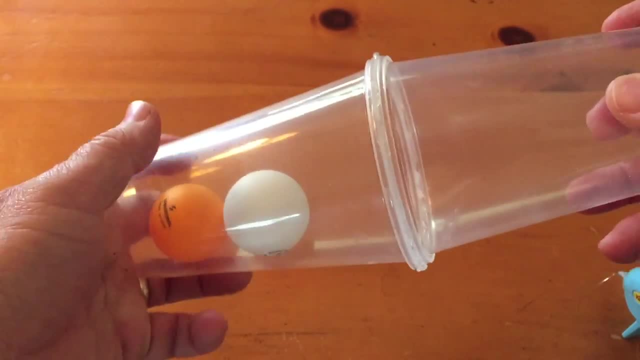 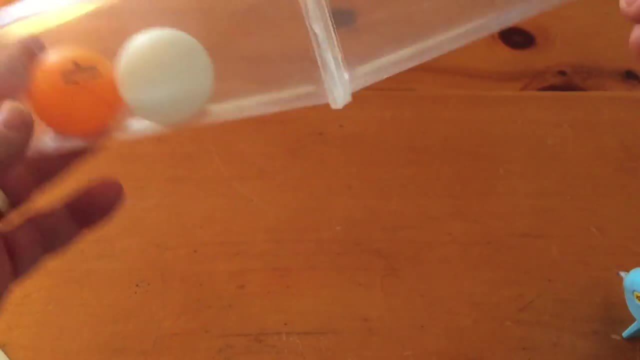 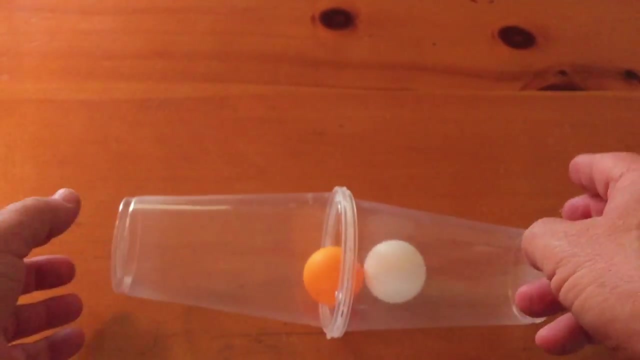 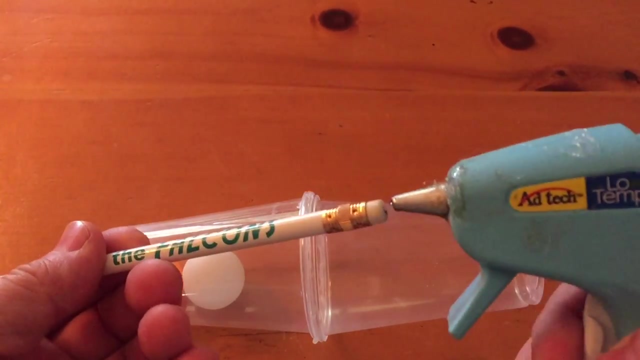 Hot glue gun. Hot glue, should you know, glue within 15-20 seconds- Varies on each gun. But once you're done, you've got your pretty much set up. You have one more piece to put on and we're going to hot glue the pencil kind of like a holder. So I check there It's all sealed up and we put the pencil right in the middle here. So put a little bit of hot glue on the eraser end, Put a whole bunch on, because you want this to really stay on. I'm going to probably have to add a little bit more than that. 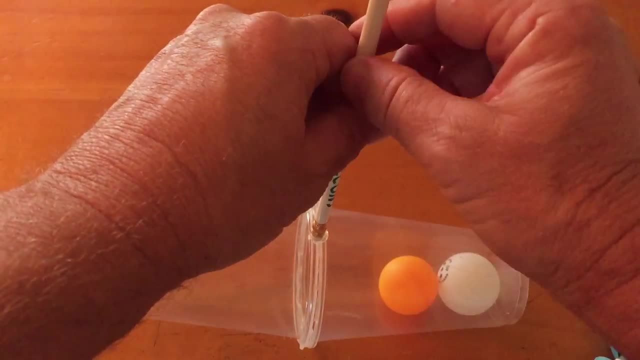 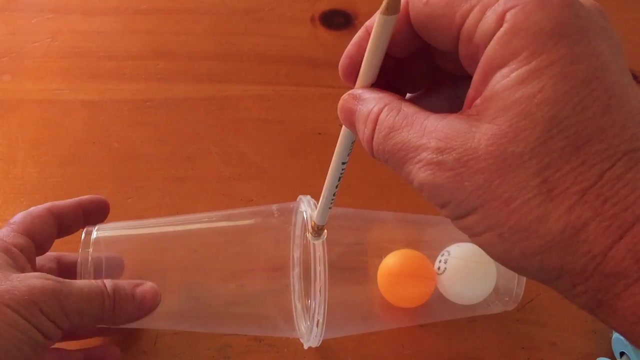 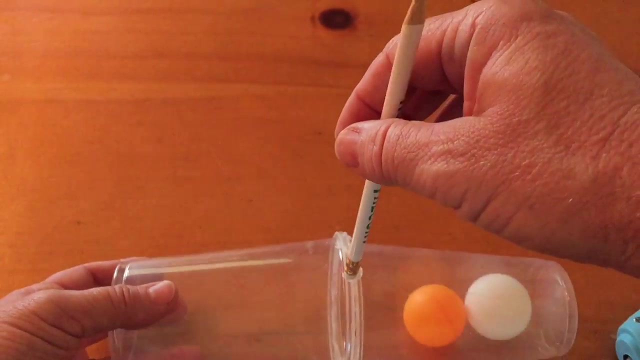 Then hold it down until it dries. It'll just take a little bit And then you're ready to go. So the object of this experiment is to separate the two balls. Put one ball on each glass. This seems tough, but if you place the glass on the table and put the balls right in the middle and just give it a spin, you'll see the spinning glass makes the balls fly towards the extreme ends, just like this. 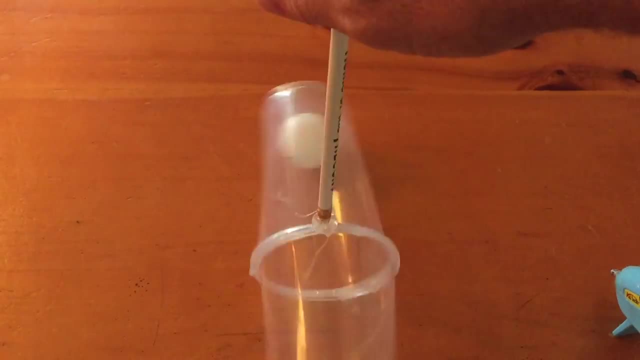 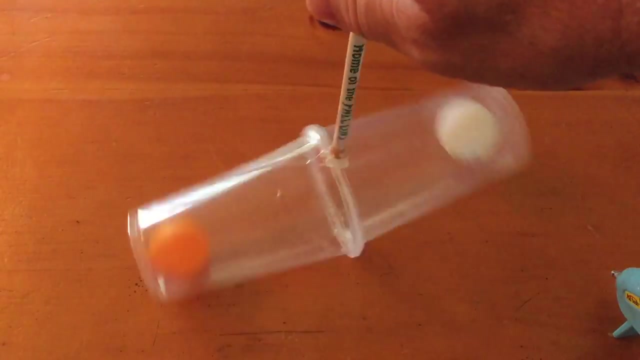 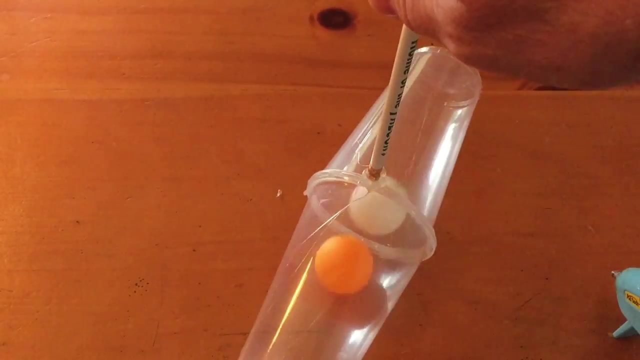 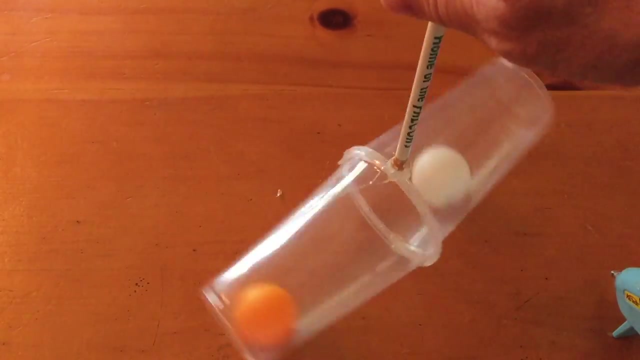 Just like when you swing an object around on a string or a rope, the object will pull outward on the string. This is called the centrifugal force. It is called by the inertia of the object where it seeks to follow the straight line of path. 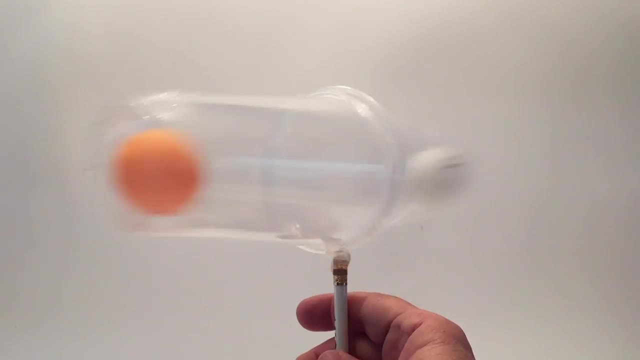 The centrifugal force is equal and opposite to the centripetal force that acts upon an object, causing the object to curve in a line Amusement park ride. This is a perfect example that it shows the centrifugal force of the roller coaster. When the roller coaster goes over that curved top of the tracks you feel the centrifugal force pulling you upward. 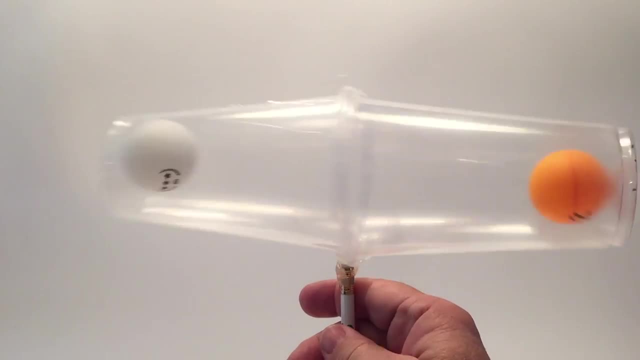 Likewise, at the lower curved part of the tracks, you feel the force pushing you downwards. I hope you enjoyed this video. Remember to click thumbs up and to subscribe, as we do a new video every day. Thanks for watching.